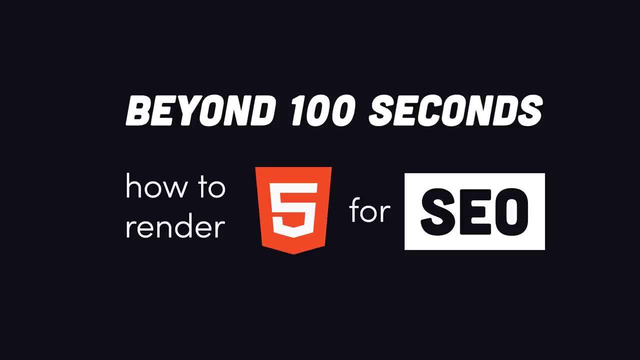 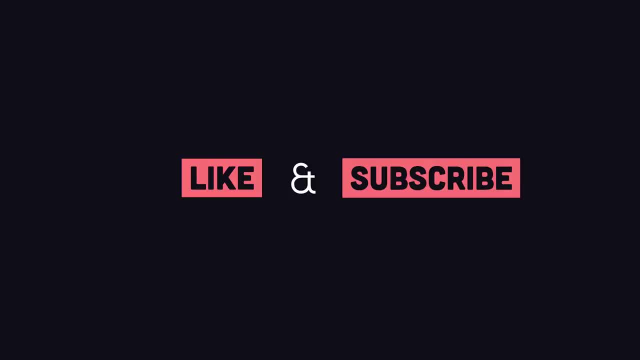 That's why today we're going beyond 100 seconds to look at the many different strategies we have to render HTML and how they impact search engine optimization. If you're new here, like and subscribe. and today I have a big announcement: My full Nextjs Firebase course is now available. 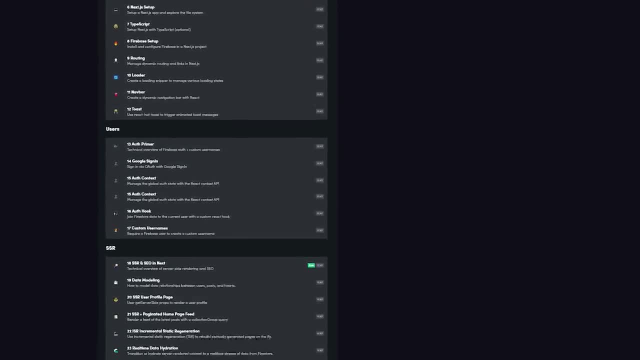 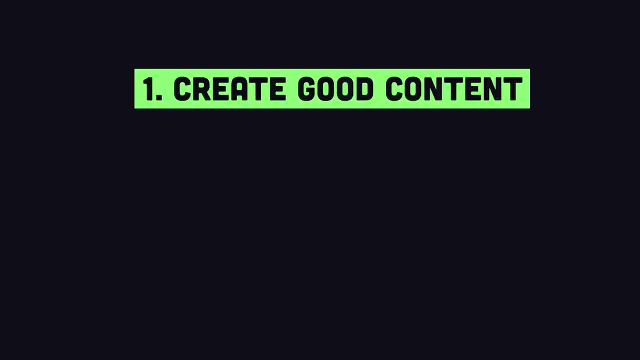 If your goal is to build a highly interactive web app that is also fully search engine friendly, then you'll definitely want to check out this course Now. the four most important rules for SEO, in my opinion, are: create awesome content. create awesome content. 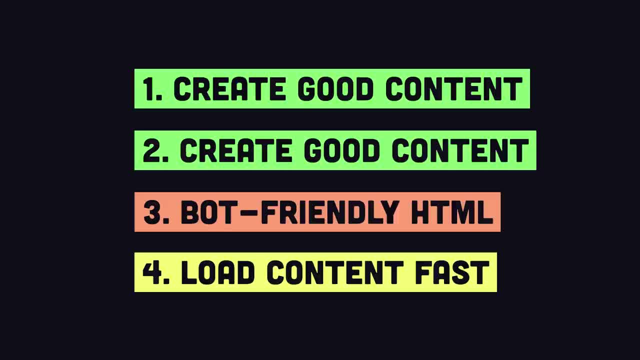 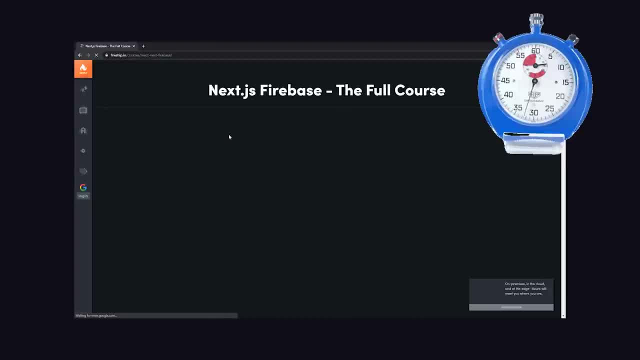 Render properly formatted HTML and load your HTML quickly. The first two rules are very subjective and depend entirely on your audience, But the general goal is that when someone clicks on a link to your site from a search engine ranking page, they should engage with your site as long as possible. 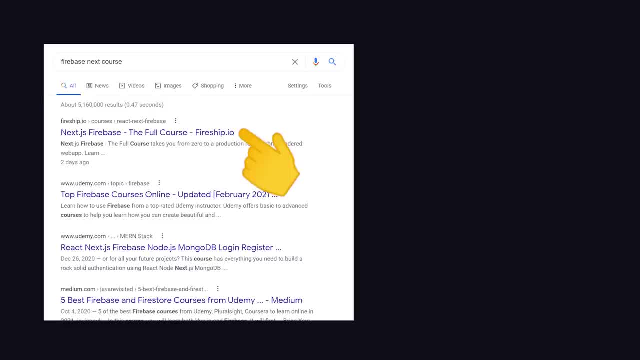 There are a few metrics that you'll want to be aware of here. The first one is the click through rate, or CTR. That defines how likely a user is to click on your link when displayed in a search engine ranking page or SERP. 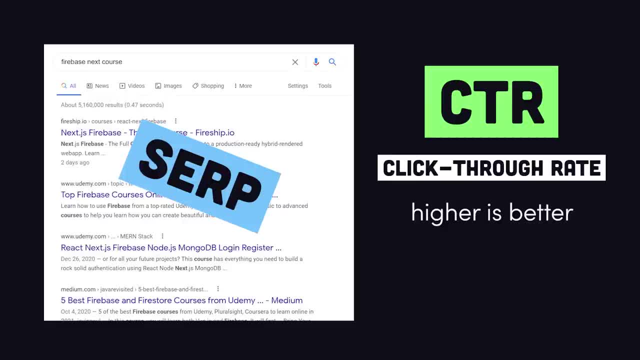 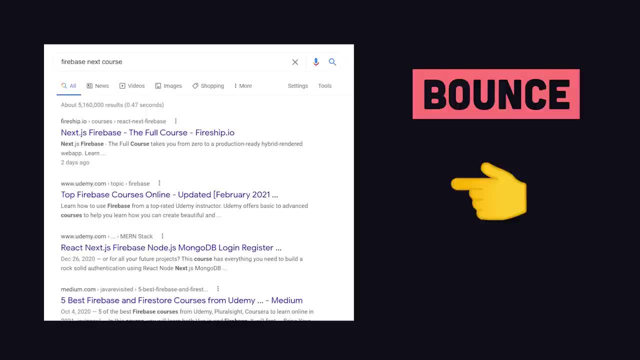 The higher the CTR, the better, And that usually means you have a very relevant title and description. Now, if a user clicks on your link and then immediately clicks the back button, that's called a bounce, And the higher your bounce rate is, the less likely your site is to rank well in the long. 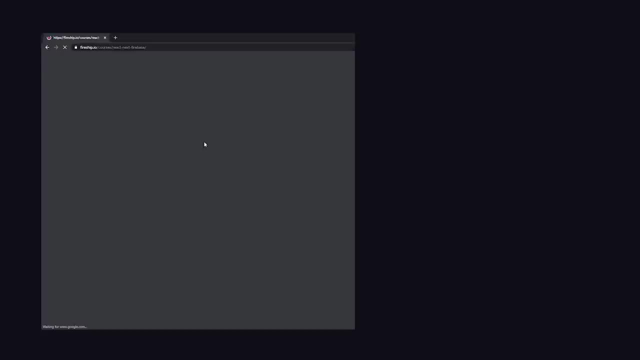 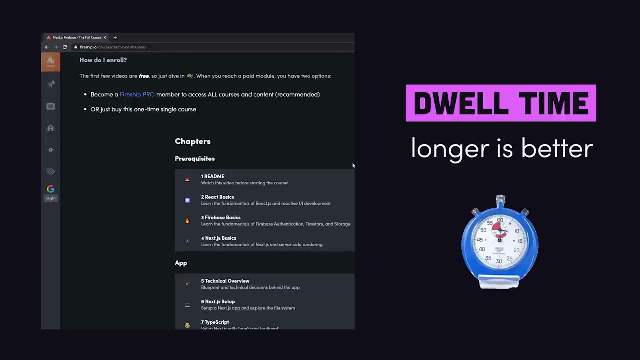 term because apparently, the content on the page is not very relevant. If the user does stay on the page, Google will keep track of the dwell time, which is the amount of time they spend there before clicking back to the search results. The longer the dwell time, the better. 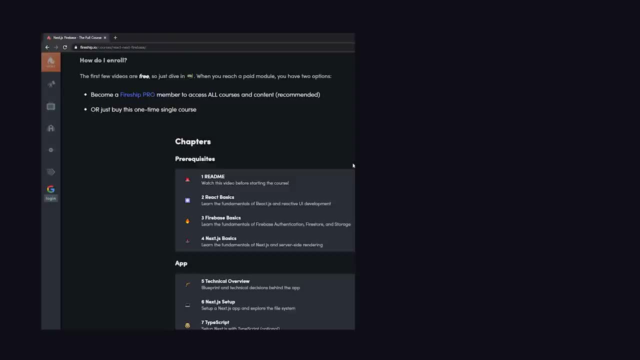 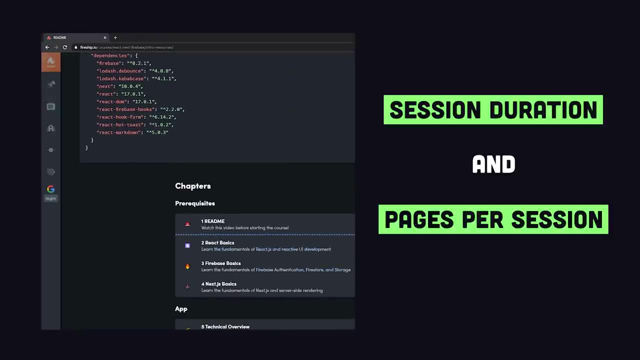 But the best possible thing that can happen is that the user never clicks back. their session will last forever And they'll never need to go to another website ever again. That doesn't happen very often, so what you keep track of is the average session duration. 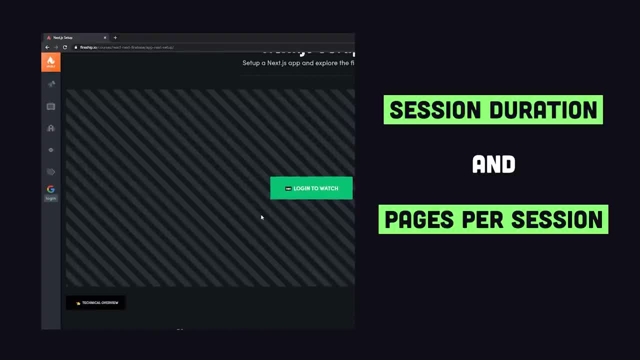 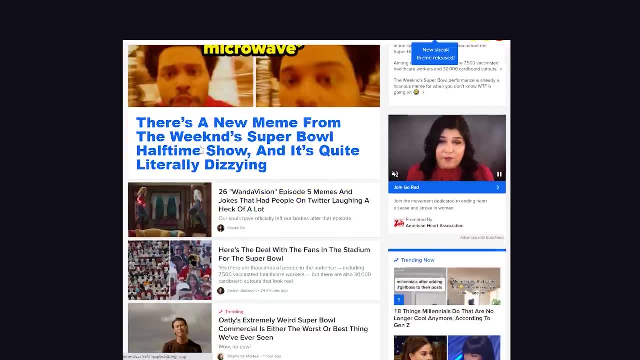 and the average number of pages viewed per session. These are metrics that you want to maximize. There's no absolute rule for creating engaging content, but the first thing the user sees should hook them in to want to read more. If you look at something like Buzzfeed, all you have to do is put an animated GIF at the 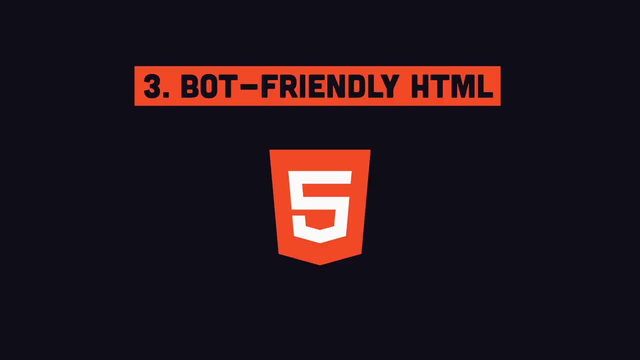 top, then maybe a few more in the body and you should be good. Let's move on to rule three, where we talk about the actual structure of the HTML. Let's move on to rule three, where we talk about the actual structure of the HTML. 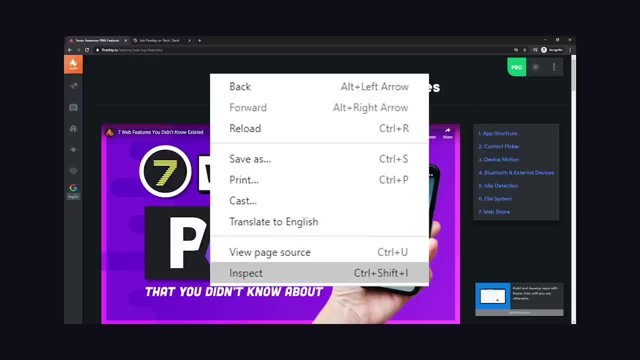 Let's move on to rule three, where we talk about the actual structure of the HTML. I'll be using my site, Fireshipio, as an example. On a lesson or article page, you can right-click and hit Inspect Element or hit Ctrl-Shift-I. 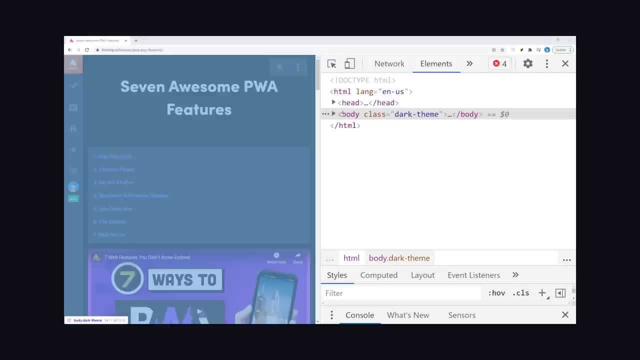 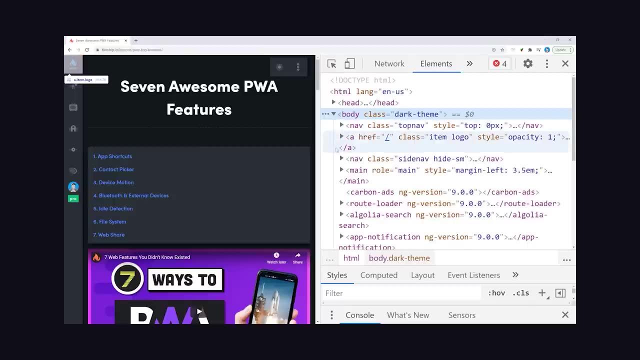 This will bring up the Elements tab in Chrome DevTools, showing you the fully rendered HTML markup. We have a head and a body. Let's go ahead and open up the body, find the main element. then, inside the main element, you'll notice we have an article. 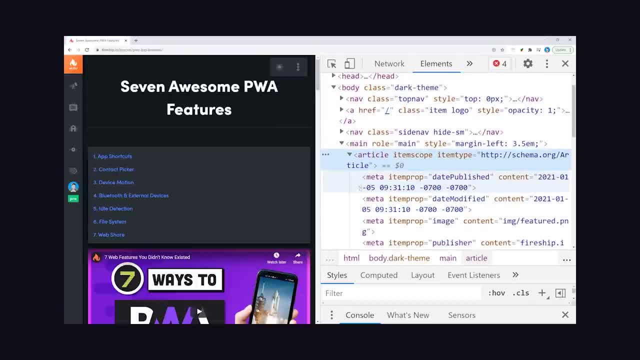 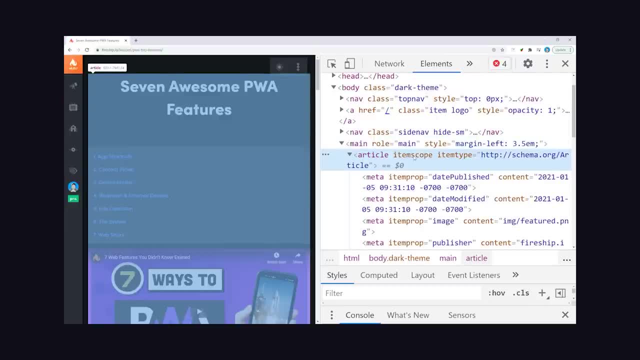 An article element has semantic meaning and, although it will never be seen by the end user, it tells the search engine. here is the main content of the page. In addition, you'll notice a couple of extra attributes here. One is item scope and the other is an item type as a schemaorg article. 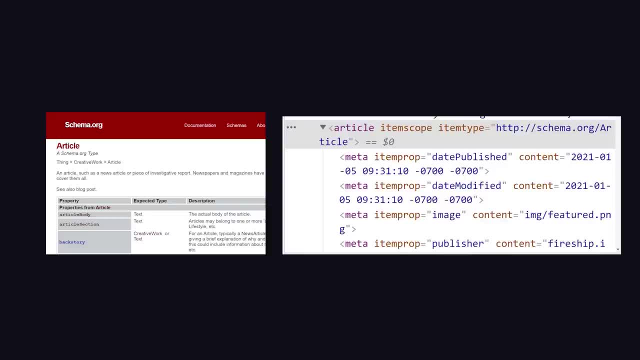 Now, it's totally optional, and whether or not it will improve your search engine ranking is debatable, But what schemaorg allows you to do is define a bunch of metadata about the actual content on your page, making it easier for search engines to interpret. 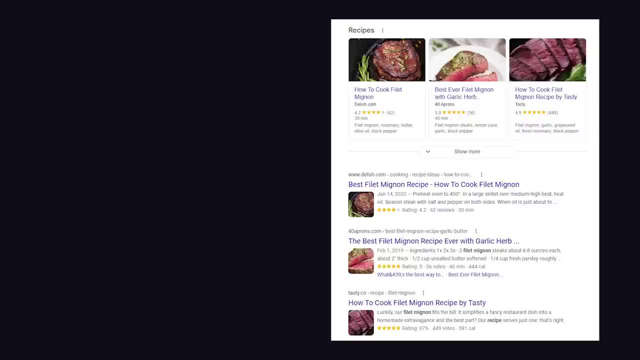 It's especially powerful if your content is something like a recipe or a star review, because Google can then take the schema data and format it properly in a certain way. So let's go ahead and do that. Let's go ahead and do that. 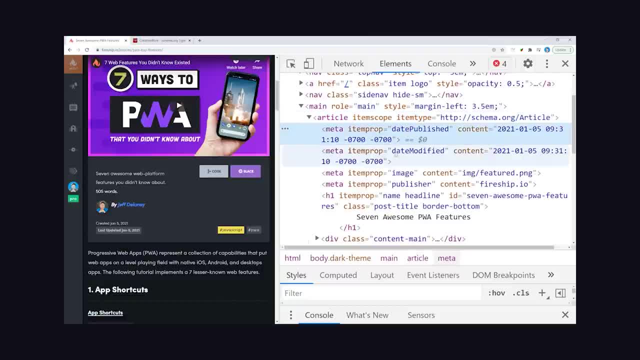 Let's go ahead and do that. So let's go ahead and do that. So let's go ahead and do that, So let's go ahead and do that Now. in this case, we have a bunch of metadata that make up an article. 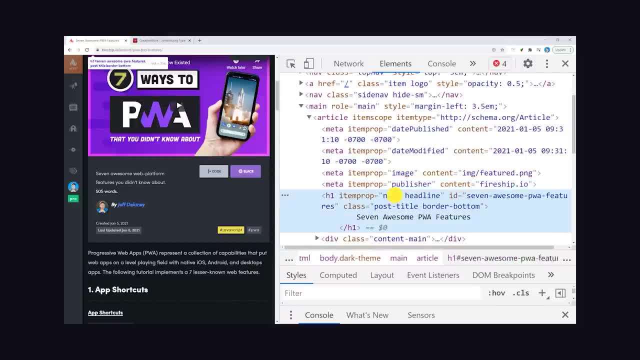 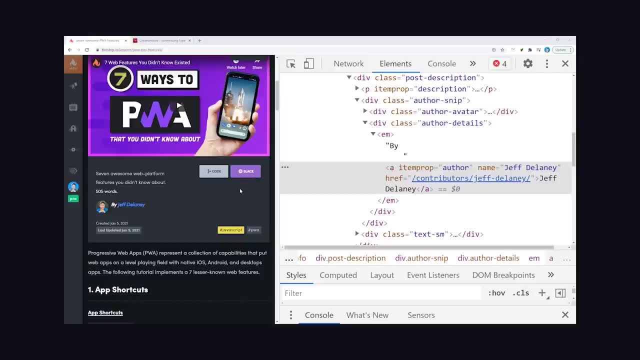 And one thing that is known to improve search ranking is when an article is written by a known author. Further down the HTML tree here you'll notice we have an item prop of author which points to the author's page. That link goes to another page on Fireshipio. 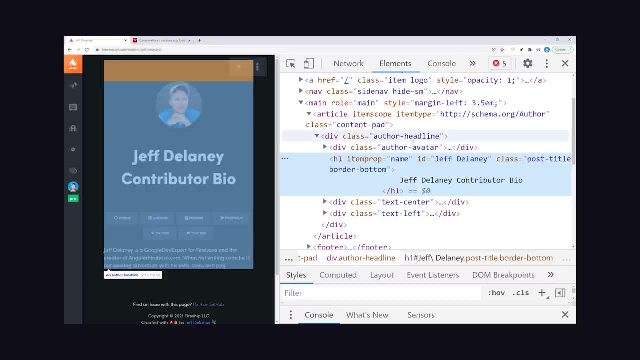 And on that page we also have an article element, this time with an item type, of a schemaorg author, along with a bunch of links that point to authoritative sites for that author. Outbound links on a page are really important Because they further signal what the page is about. 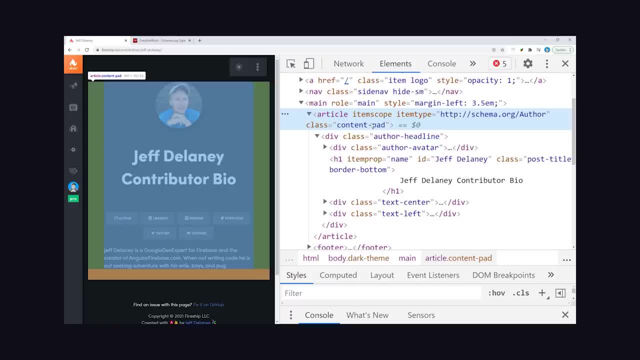 In this case, Google will first crawl the article, then crawl the author's page, then crawl these other sites to understand who that author is. A good strategy is to use outbound links to other really good sites that are related to the content on a given page. 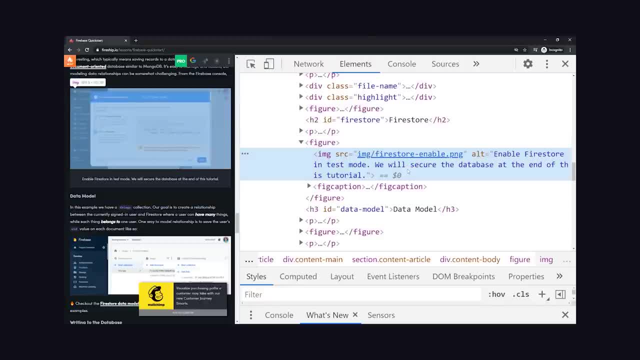 Now, in addition to schemaorg, there's other ways you can add metadata to your content, And this can be very important for SEO and also accessibility. One of the most fundamental techniques is to add an alt attribute to images, which is basically just some text. 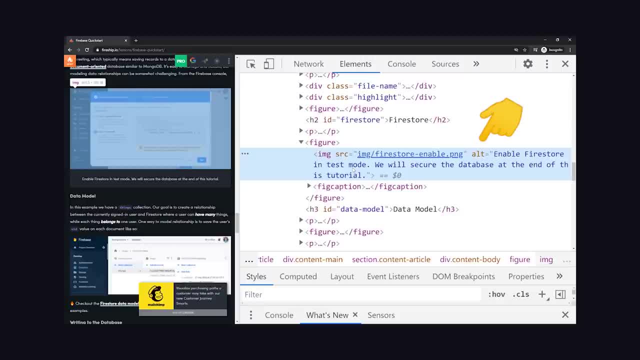 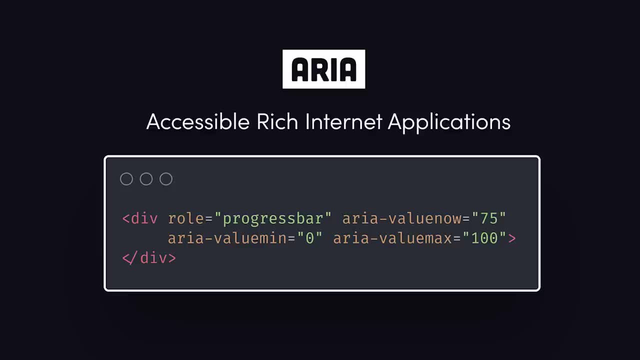 It's a text that describes the image. This metadata can be used by search engines and also by screen readers for those with disabilities. For other elements that are a little more complicated, like a progress bar, for example, you can use ARIA attributes, which stand for Accessible, Rich Internet Applications. 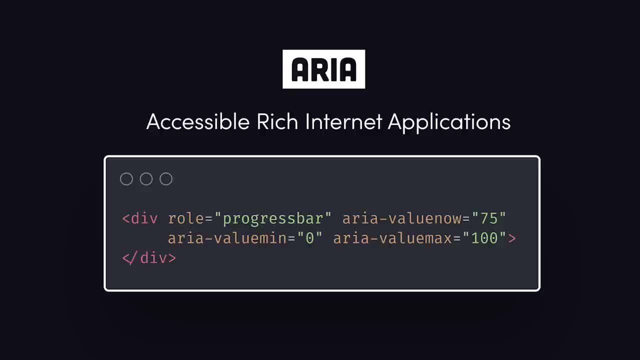 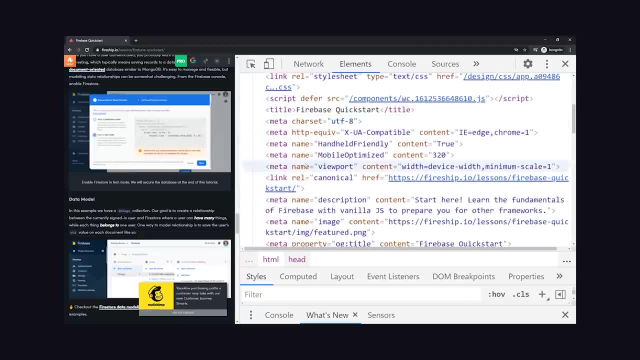 And they help provide additional meaning to highly interactive widgets on the page. At this point, we've only been looking in the body of the document, But the head of the document contains all kinds of useful metadata for SEO. Most importantly, this is where you have the title. 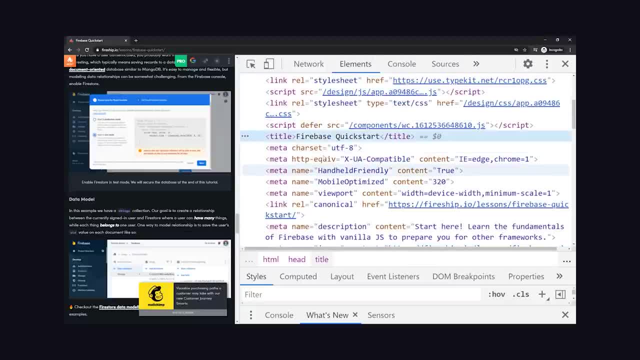 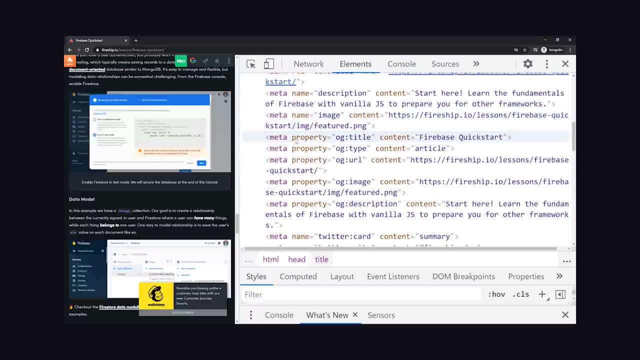 You should choose your title carefully, because it's displayed in a SERP page and will ultimately control your CTR rating. In addition to the title, you may also want to have metatags here which define things like the description, featured image, author, canonical URL and stuff like that. 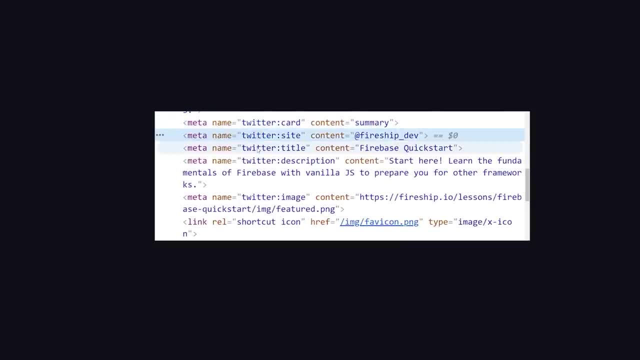 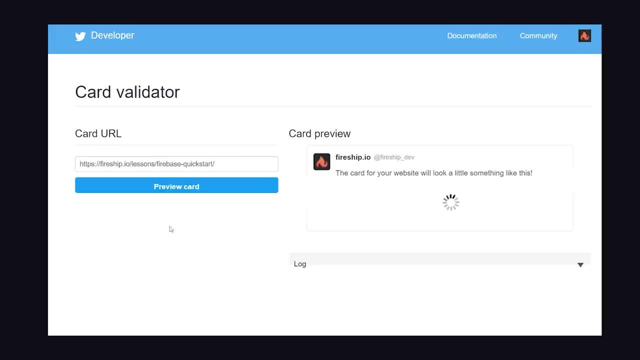 These metatags are also essential if you want your content to be shared on social media sites like Twitter or Facebook. When you post a hyperlink in social media, it fetches that page and looks for the metatags to understand what image and title to display there. 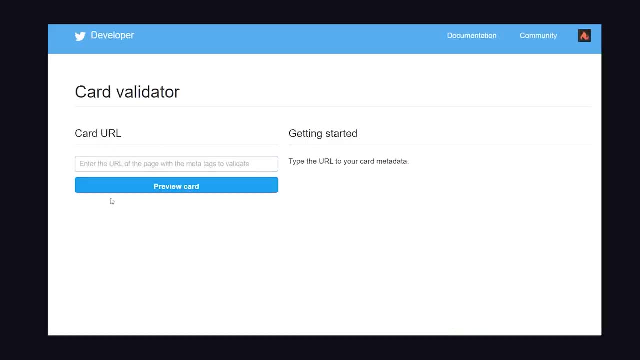 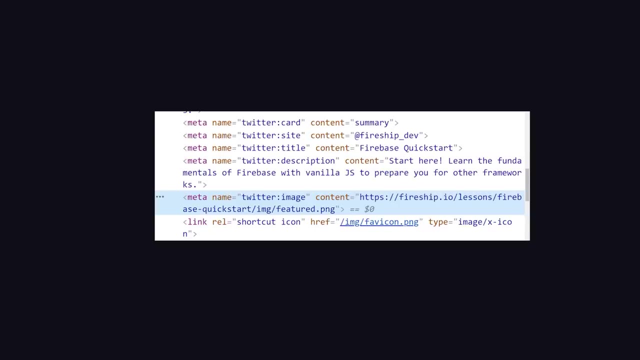 If you want to see how your site's doing right now, you can post a link into the Twitter card validator and it will tell you whether or not it can use your current metatags. So that gives you some things to think about when it comes to the actual structure of your 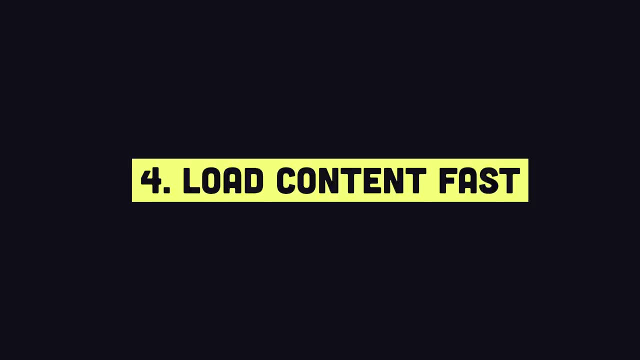 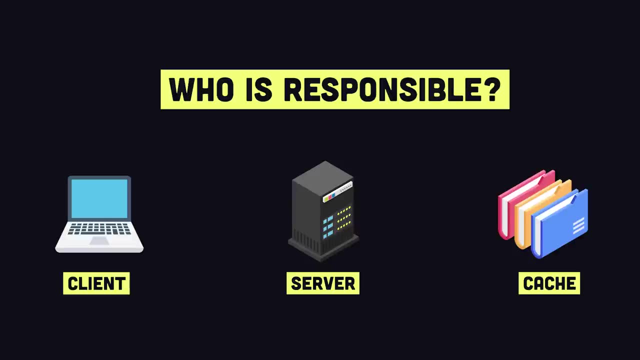 HTML, But the bigger question is: how do you render that HTML, Or, in other words, what part of your tech stack is responsible for generating the actual HTML markup that is received by a bot or end user? There are three fundamental ways to render HTML. 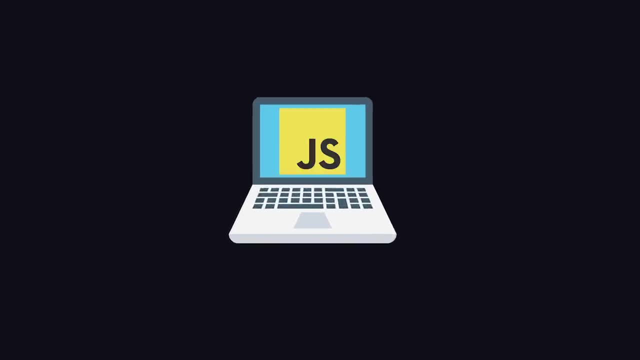 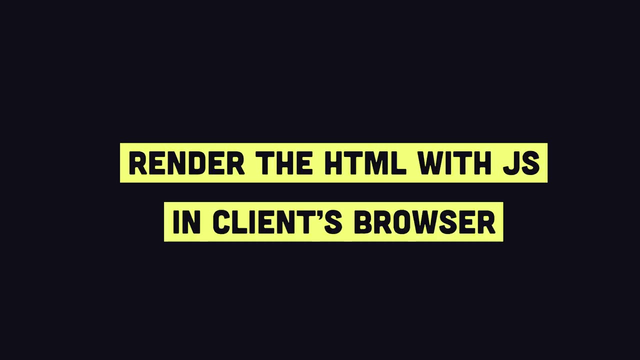 The first one we'll look at is client-side rendering. If you're building an app with something like React or Angular, the default mode is client-side rendering or a single-page application. On the initial page load, the user gets a shell of HTML without any meaningful content. 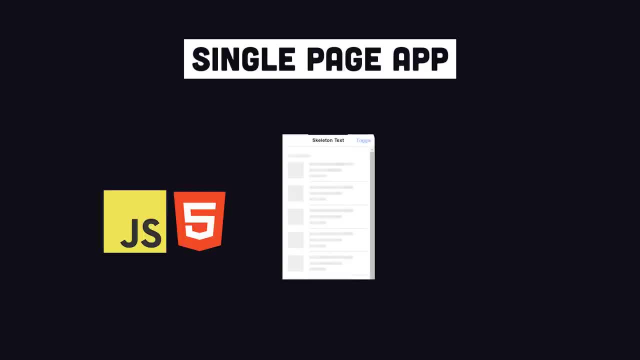 The JavaScript code then bootstraps, then asynchronously fetches any additional data needed for the UI. Apps like this are great for interactivity because it gives the end user an app-like feel, similar to what you'd expect on iOS or Android. The problem is that because the initial HTML is just a shell, search engines may have a 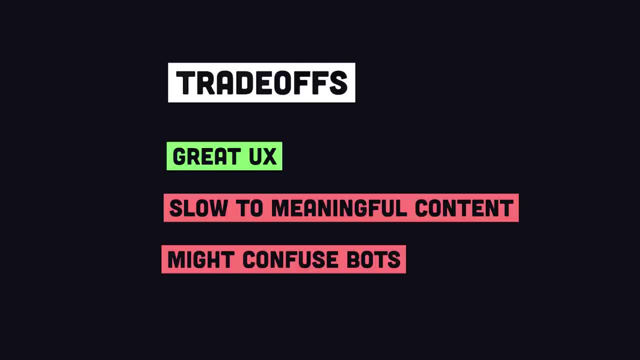 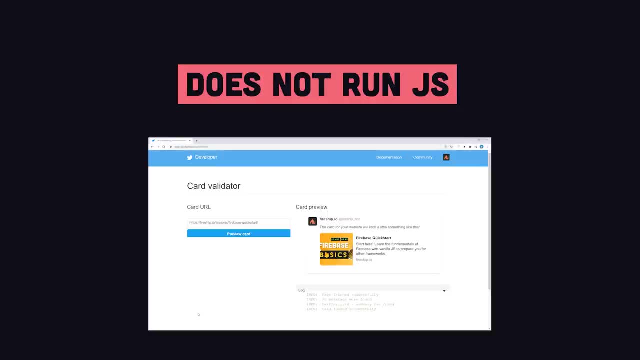 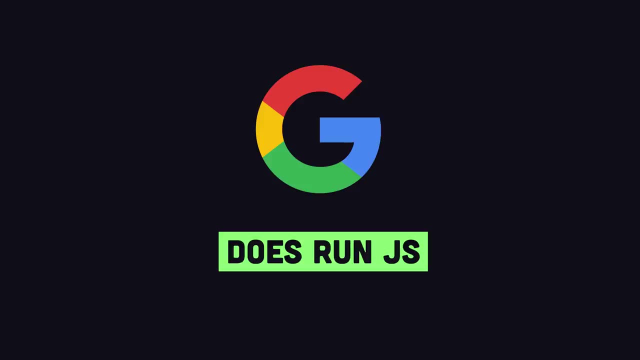 hard time understanding it. If you take a link generated by JavaScript from a single-page application and post it into Twitter, you'll only see the initial shell. You won't see any additional meta tags that were generated by JavaScript after the fact. That's not great for social media, but Google, as a search engine, is able to index client-rendered. 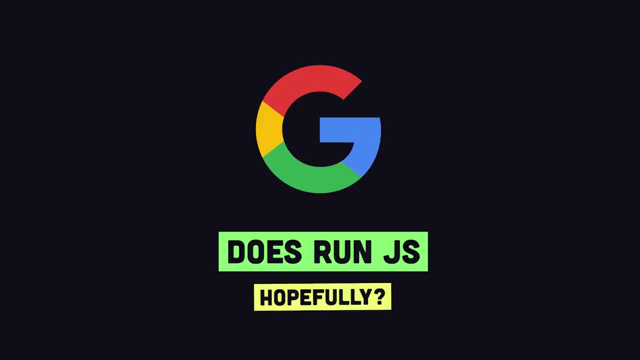 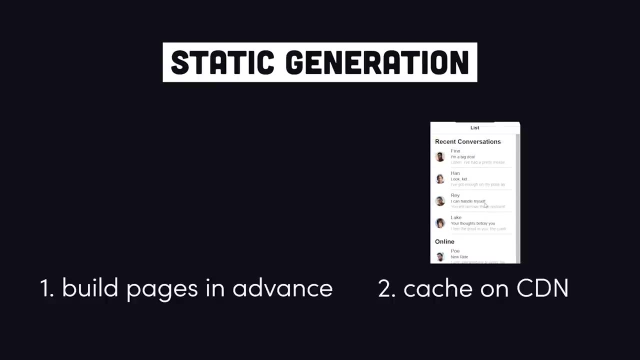 apps, But the reliability is questionable And personally I wouldn't trust client rendering if SEO was a business-critical requirement. So another option is to prerender or statically generate HTML. Let's imagine your web app has a hundred different routes or pages. 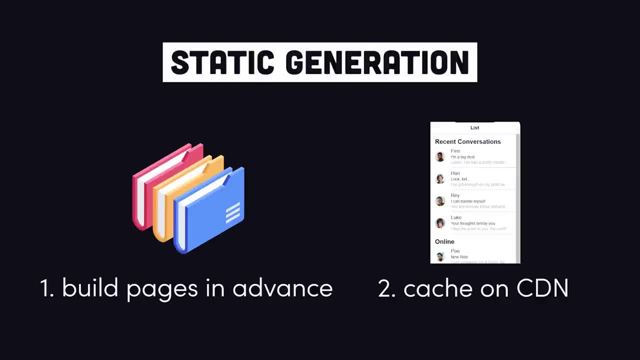 Instead of sending a shell down to the user, we could generate all the HTML for those pages in advance, then upload the static files to a storage bucket that could be cached on a global CDN. So the first thing the user sees is fully rendered content. 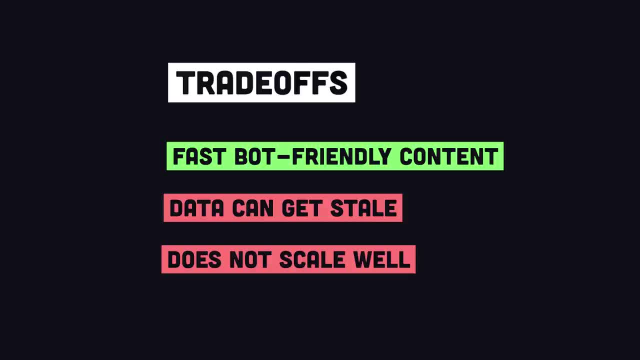 Then the JavaScript loads after that and makes the page fully interactive. That's great for SEO, because bots get fully rendered HTML and they can easily interpret the content on the page. It's also highly efficient because if you're fetching a lot of HTML, you're going to need 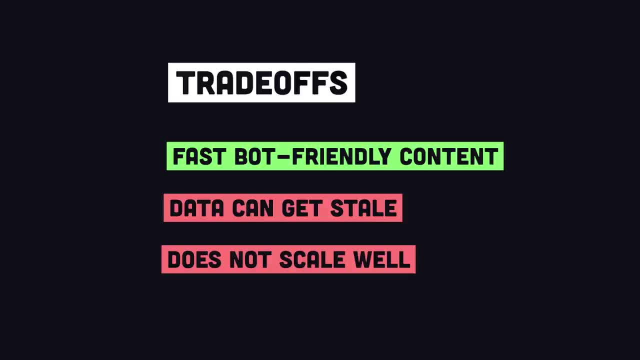 a lot of HTML. If you're fetching data from a database, you only have to do that once at build time. Then you can cache the page on a CDN and serve it to millions of people without having to re-fetch your data. The trade-off with this approach, though, is that the data and the pre-rendered content 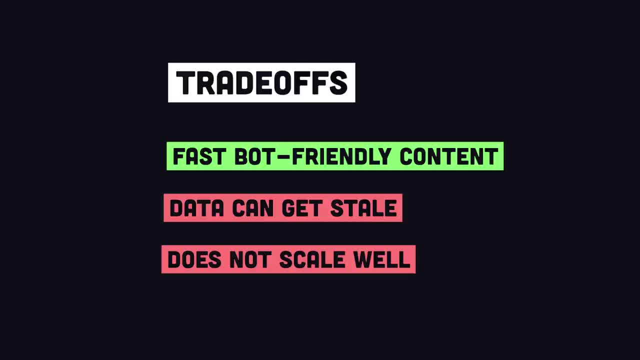 can become stale, which means bots will be getting outdated information until you rebuild and redeploy the entire site. That's no big deal if you have a few hundred pages, that don't change very often. But if you have millions of pages with highly dynamic data, then it doesn't really scale. 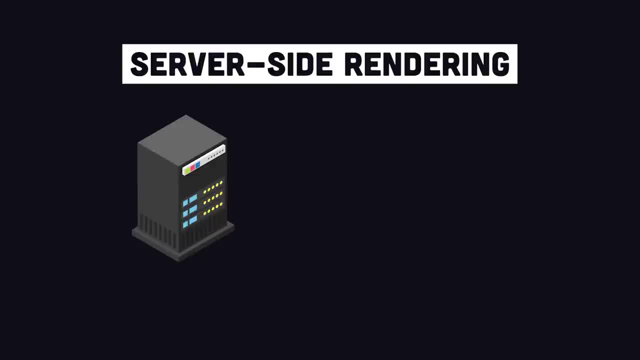 And that brings us to option number three: server-side rendering. Let's take a look In this paradigm: when the user makes a request to a page, the HTML is generated on the server. This is also great for SEO, because bots get fully rendered HTML on the initial request. 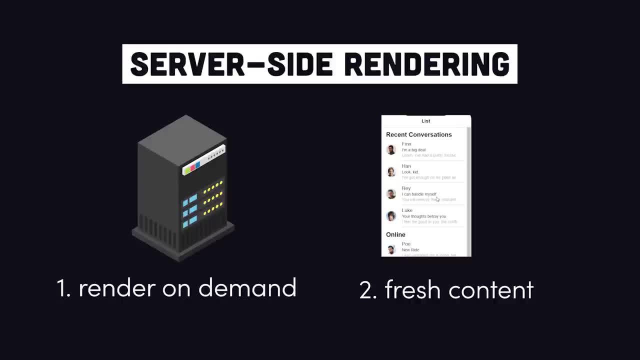 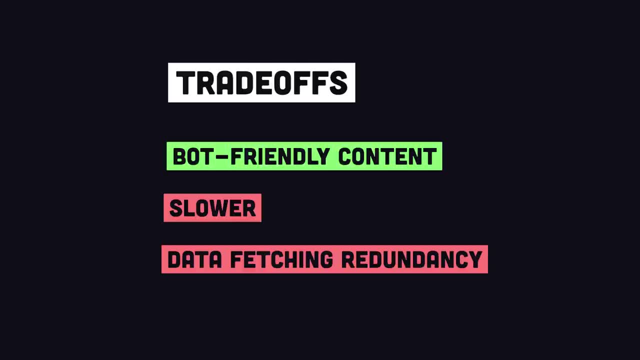 In addition, the data will always be fresh because you're making a new request to the server each time. But the drawback here is that it's generally less efficient. You might be fetching and rendering the same HTML over and over again. It is possible to do server-side caching, but that's not as efficient as edge caching. 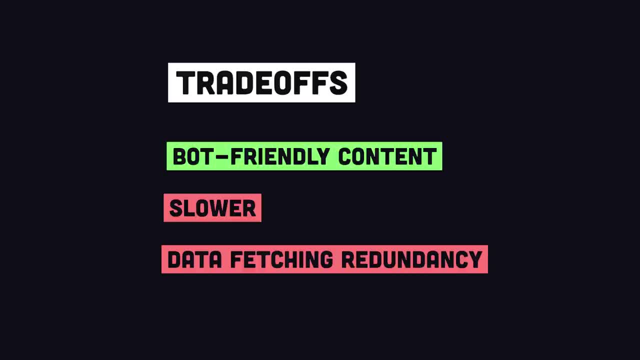 on a CDN and will cost a lot more to operate at scale. And if things aren't cached efficiently, that means a slower first time to meaningful content, which can negatively impact SEO. So basically, between these three methods we have a trade-off between data freshness. 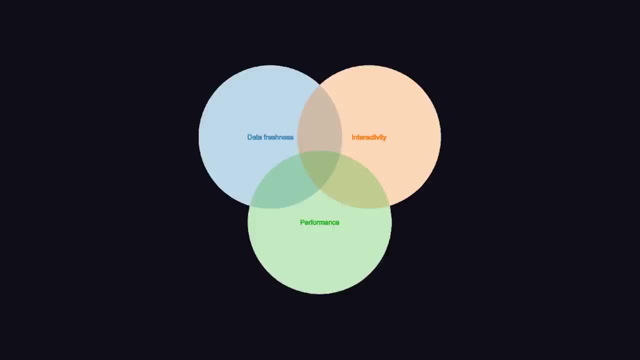 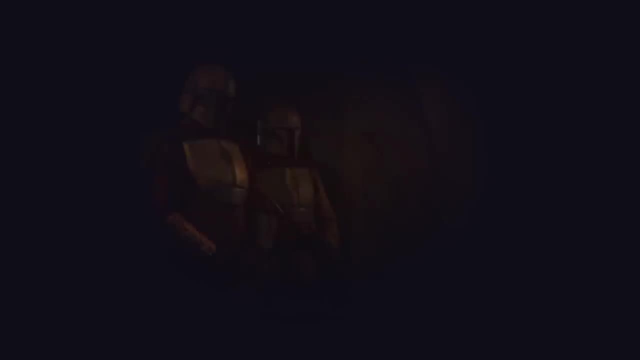 performance and client-side interactivity. But what if there is a way we could have our cake and eat it too? allow me to introduce you to incremental static regeneration. This is the way. This is the way. This is a new form of rendering available in the next JS framework.